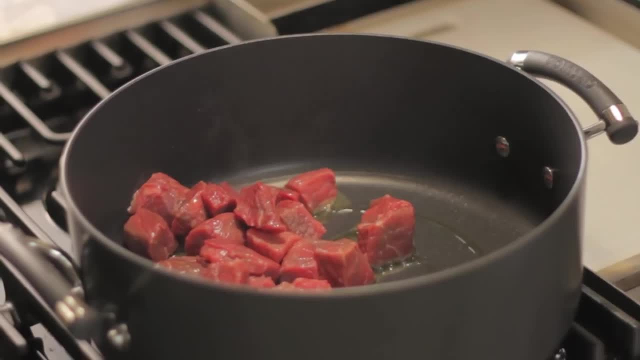 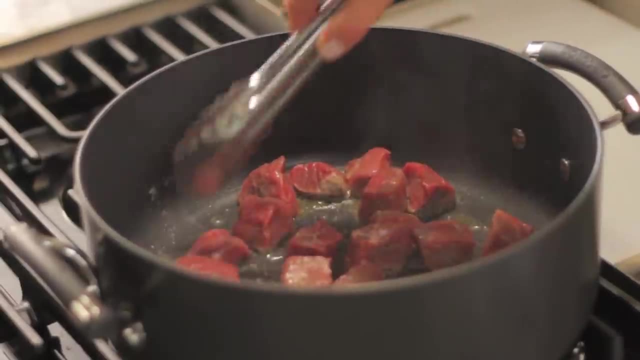 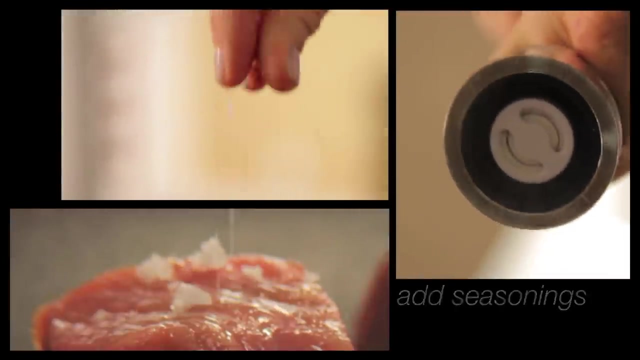 meat to brown it. Browning the meat is where the rich flavor of the stew begins. Overcrowding the pot will cause the meat to steam rather than brown, so work in batches that fit comfortably in your pot. Add a small amount of salt and pepper to the meat as it cooks, while frequently turning for even browning. 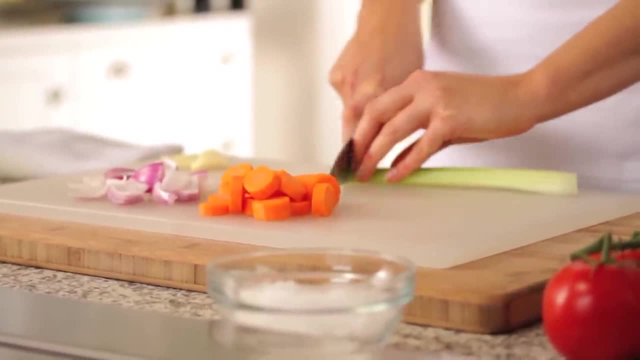 After all, the meat is browned and removed from the pot, add flavorful aromatics such as chopped onions, carrots and garlic. The meat is very tender and is a perfect substitute for a thick and and garlic, and cook for about 10 minutes until the vegetables are soft. 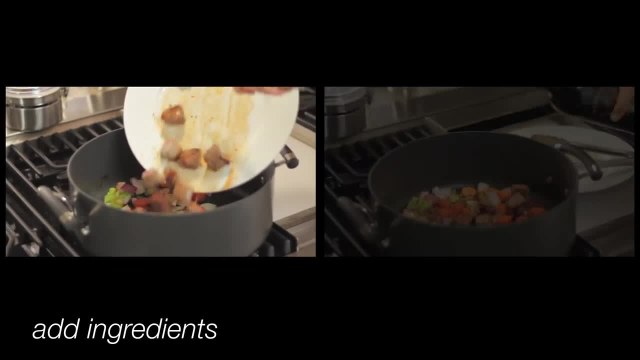 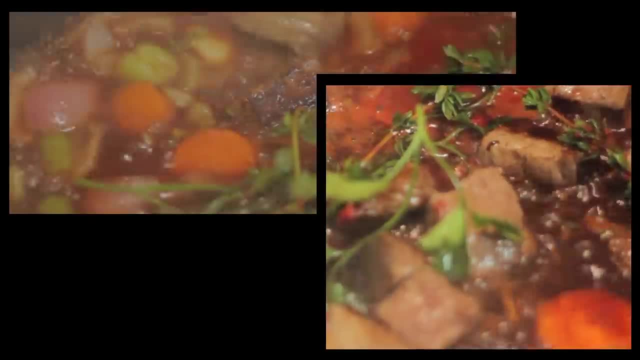 Next, add the meat back into the pot along with liquids like wine and broth and any other ingredients called for in your recipe. Bring it to a simmer and cover the pot. Cook the stew on the stovetop or in the oven. 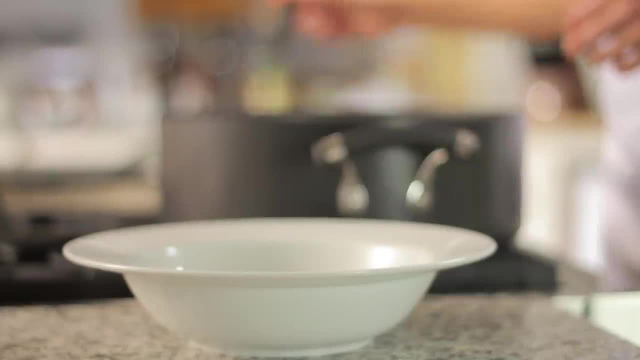 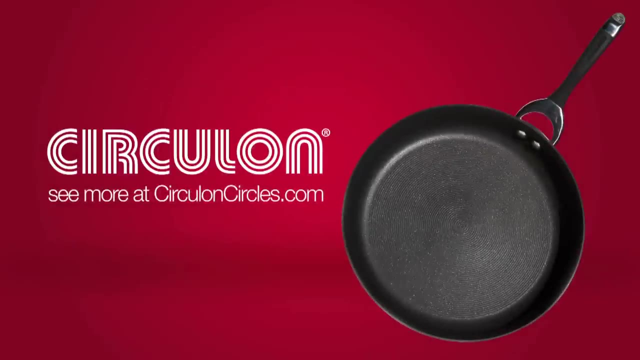 as called for in your recipe, for about one and a half hours, until the meat is tender. If you like this recipe, please share it with your friends and subscribe to our channel. 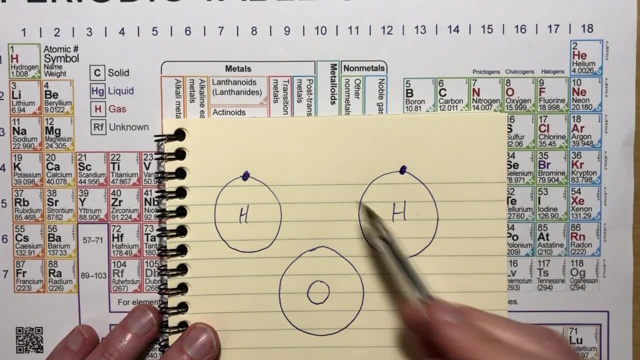 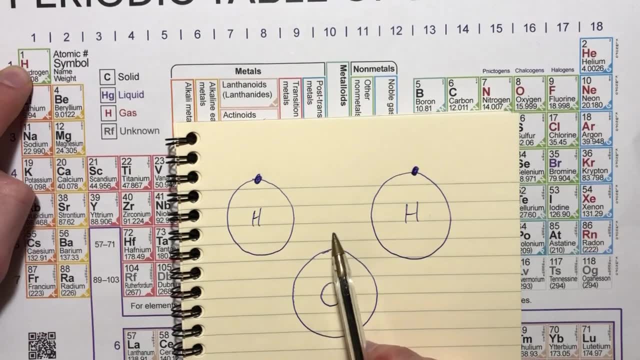 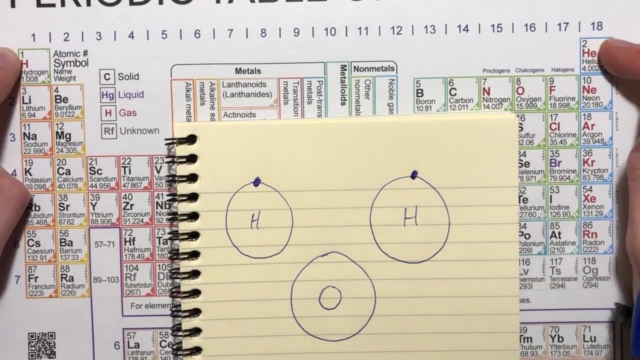 Let's have a look at the covalent bonding that takes place when hydrogen and oxygen come together to make water, H2O. So I've drawn my two hydrogen atoms with their single electron in their only shell. Oxygen, on the other hand, has an inner shell with two electrons and then another shell with one, two, three, four, five, six. 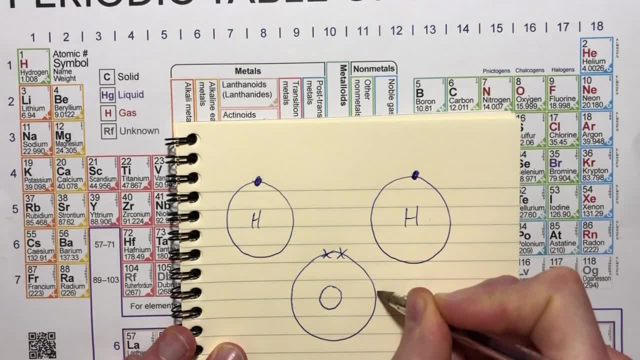 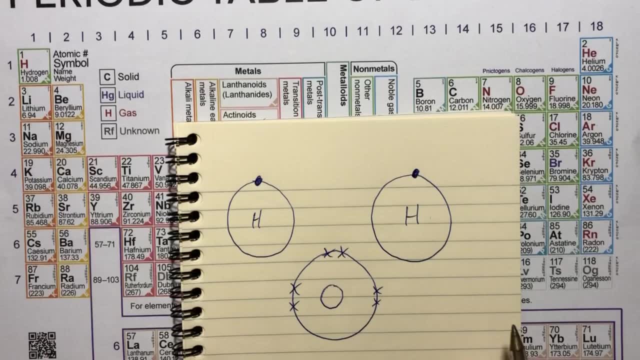 I'm only going to draw the outer shell. One, two, three, four, five, six. It doesn't actually matter where you draw them, It's just to make the diagram look nice. And now again, the same rule is: they want to get a full outer shell. 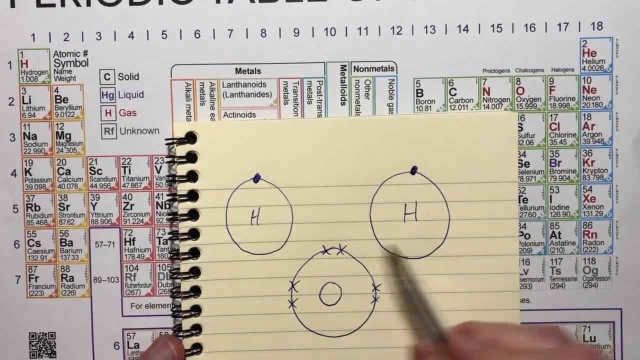 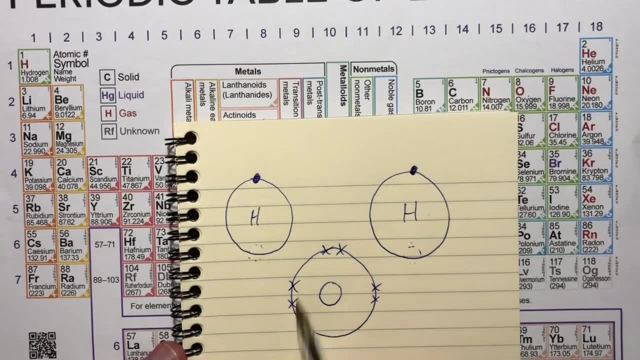 Remember, the first shell can only hold two electrons. So these two hydrogens will be happy if they can just add a single electron here or here to their shells and then they'll be full. Oxygen needs another two. It needs another two to fill its shell because its shell is the second shell.